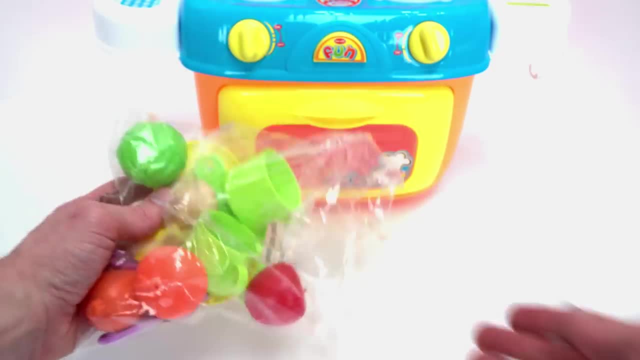 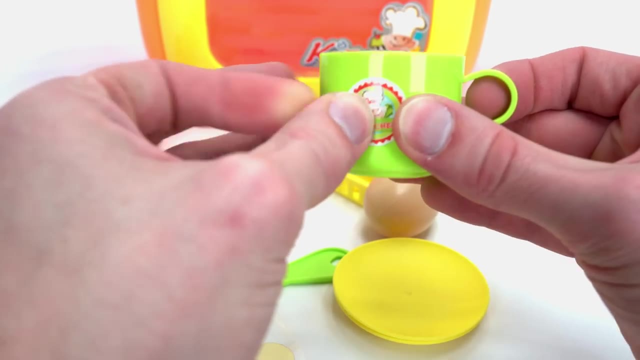 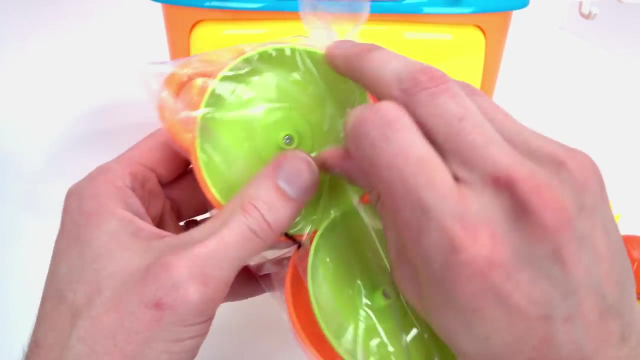 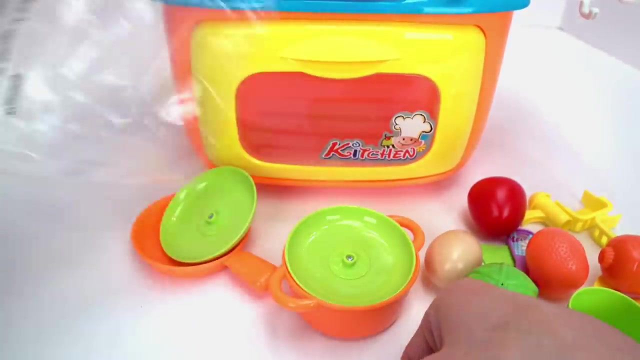 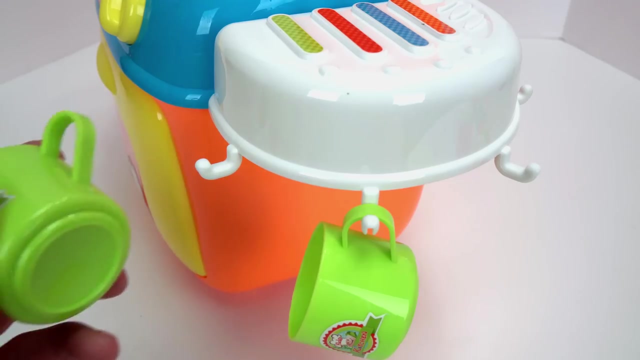 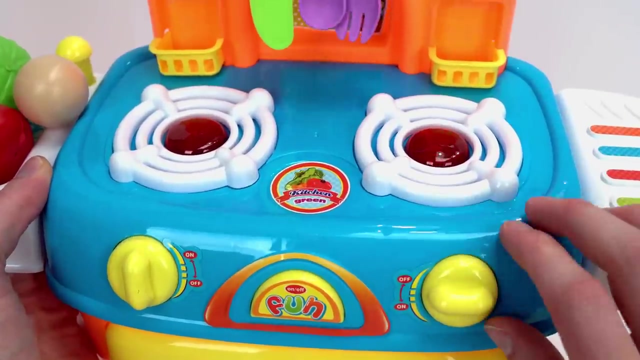 Some of these get stickers too. Now for the pot and pan. We can hang the cups like this, And the silverware too. I want to see what the stove does. Cool. How about this one, And this one, And this one. 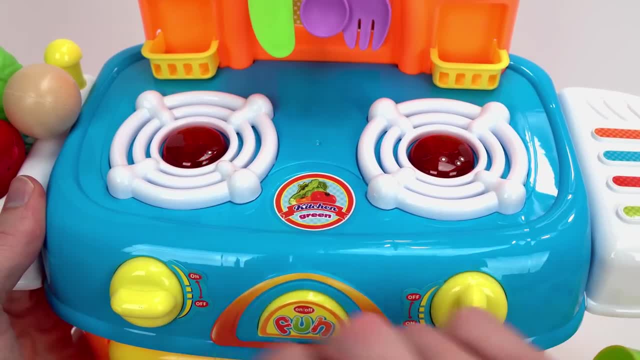 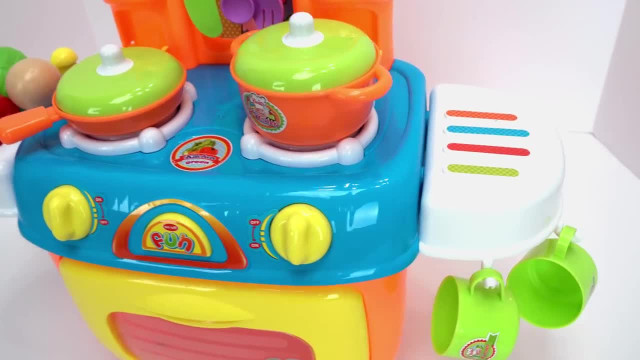 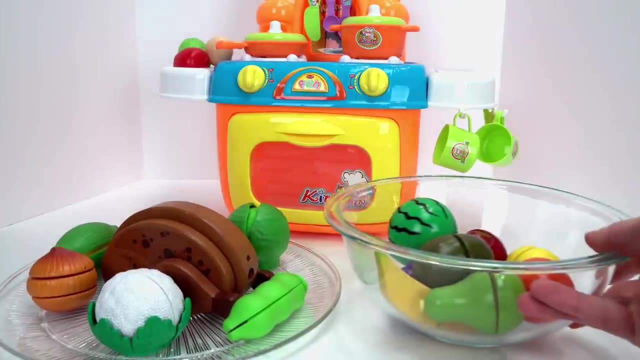 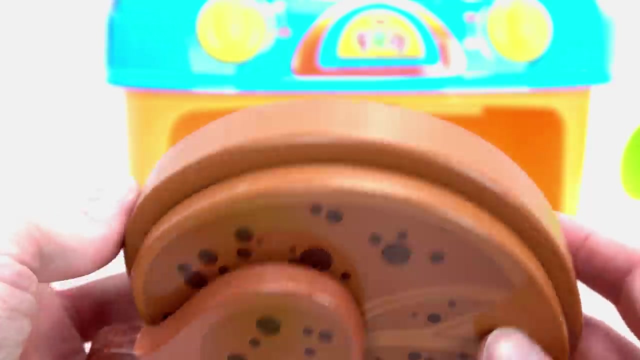 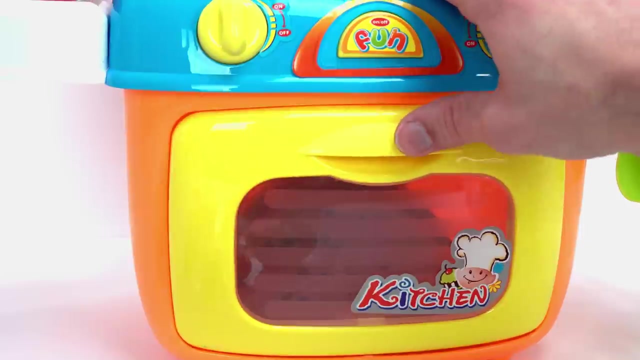 This is a super cool looking playset. Let's start cooking. Here comes the food. This is a chicken. Let's bake it in the oven. Here it goes. While we wait for that to cook, let's make a vegetable stew. 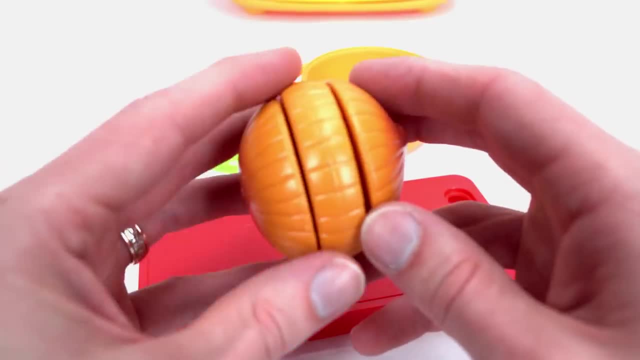 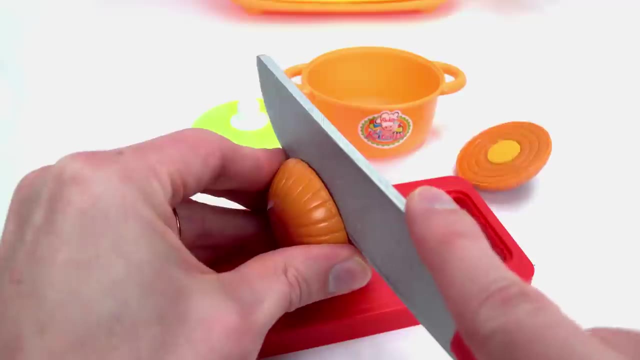 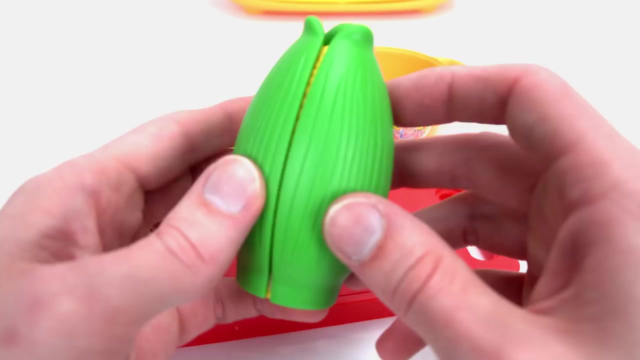 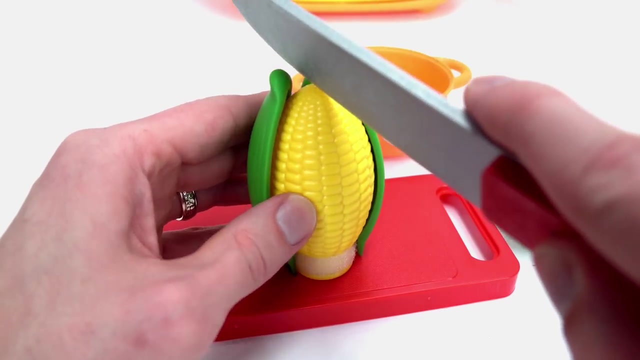 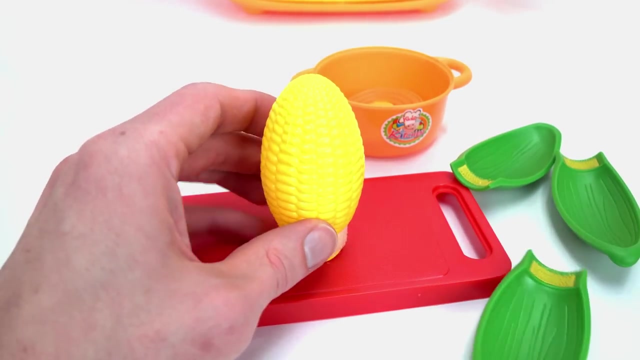 Here is an onion. We need to cut it because we only need one slice for our stew Into the pot. This is corn. We'll need to peel the husk off. One, Two And three Into the pot. it goes Now for some cauliflower. 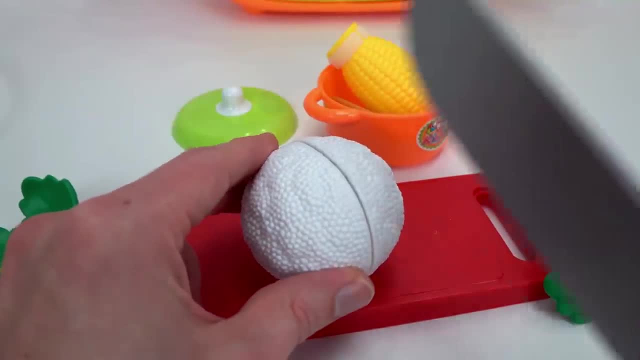 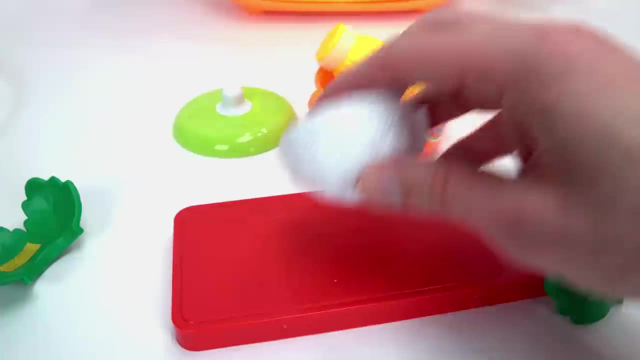 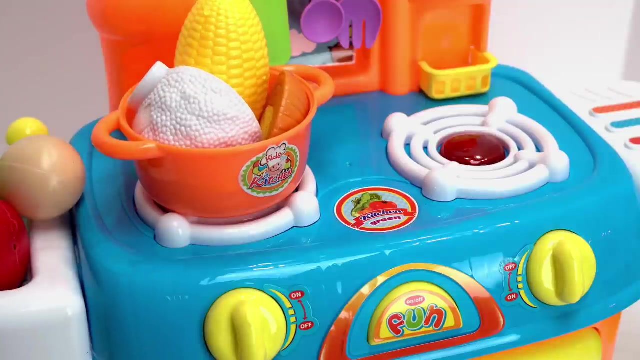 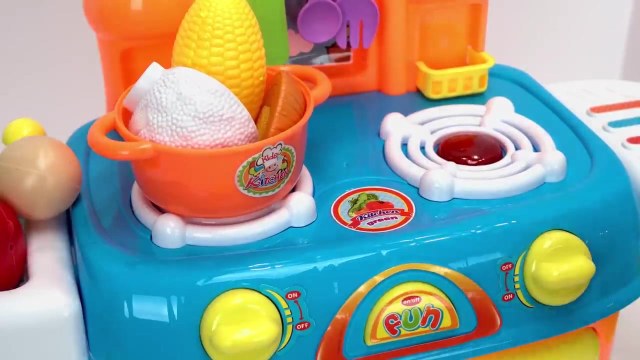 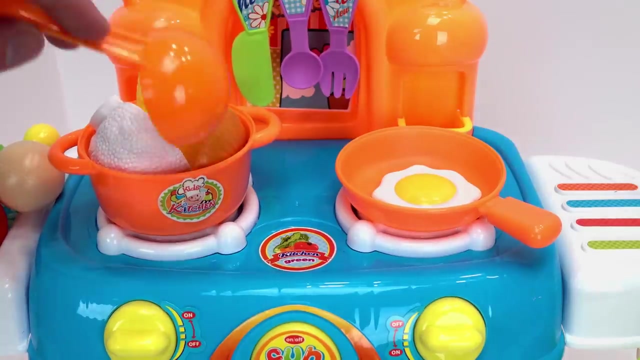 We only need half, so let's cut it, Add some water and start cooking our stew. Let's use this other burner to fry an egg. We'll need the frying pan and an egg. I think we need to stir the stew. The egg is done. 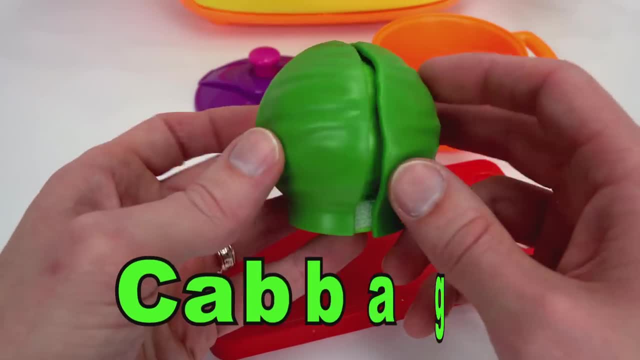 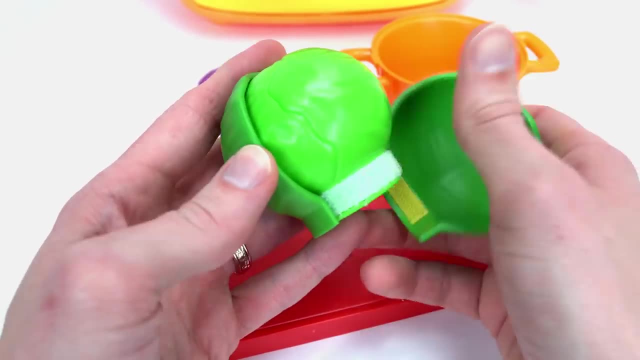 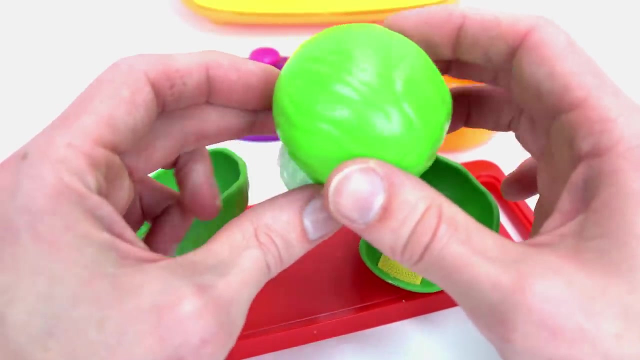 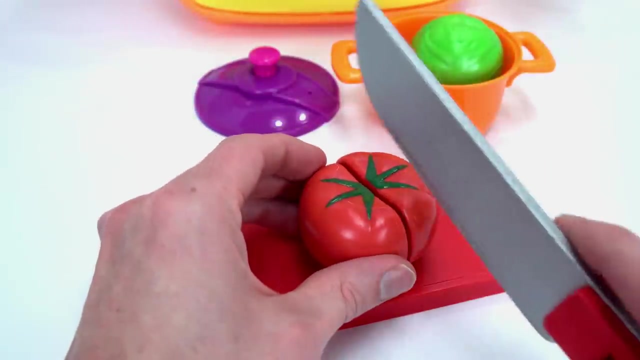 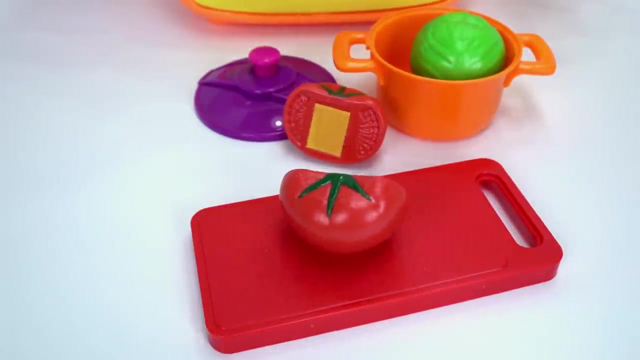 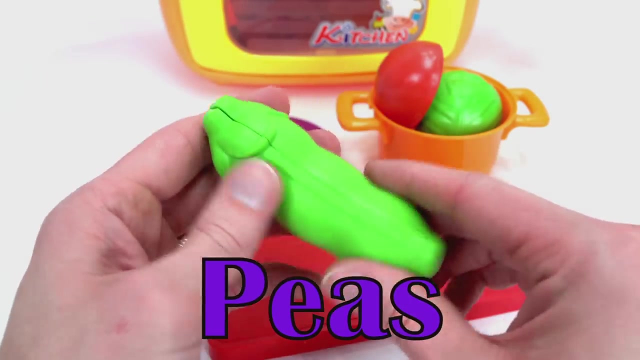 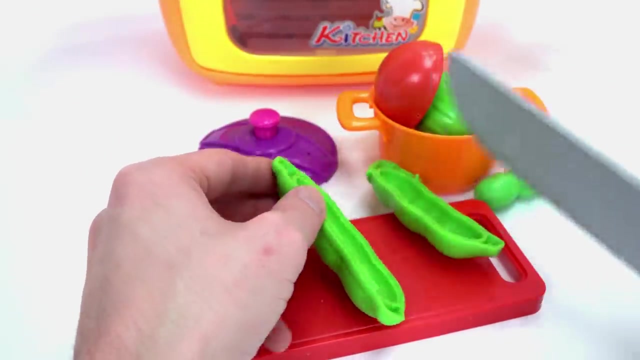 Look how yummy it turned out. Here we've got a cabbage- It looks so fresh. And here's a tomato. Let's add half of it to the pot. And now some peas. Let's split the pod and add the peas to the pot. 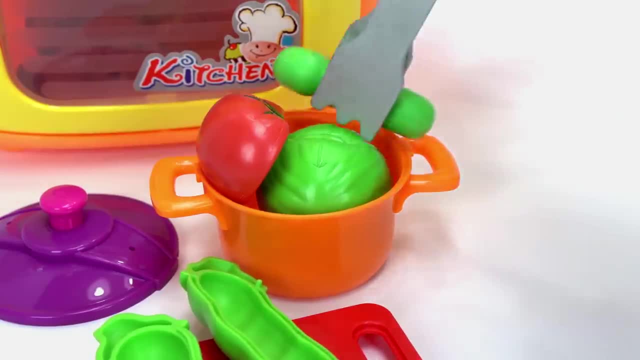 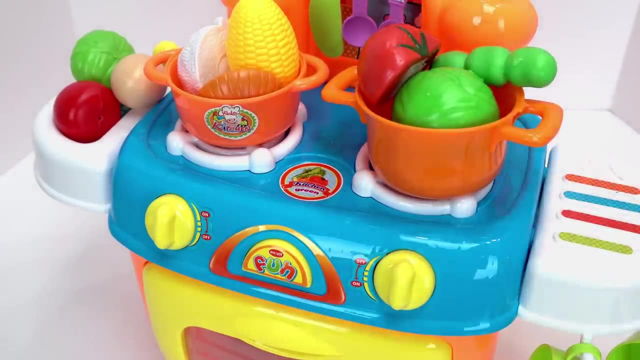 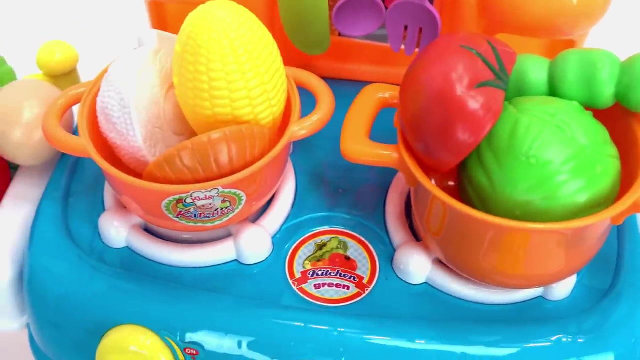 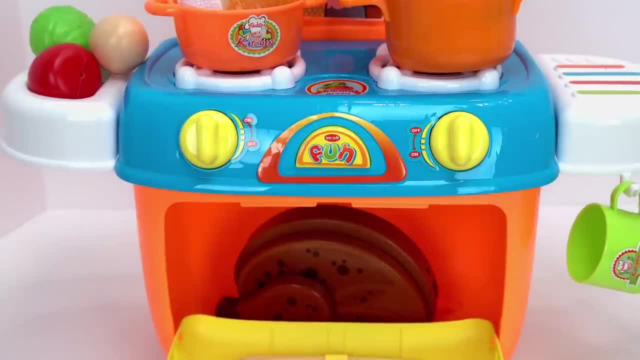 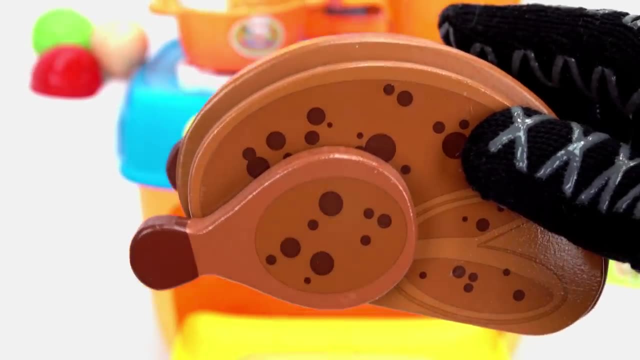 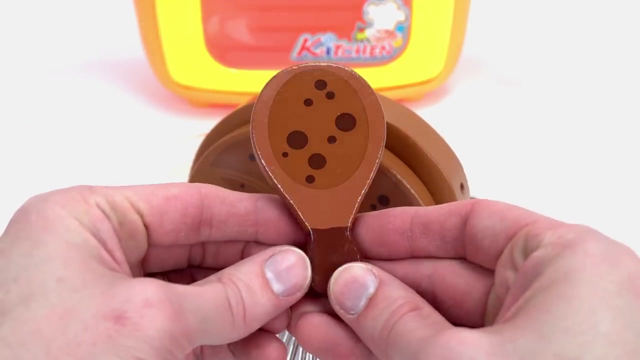 Oh, the chicken's done. It's going to be hot, so we've got to be careful. It turned out perfectly. Let's cut the chicken. Here's a drumstick. Here's a stick. Here's a stick. The nuts have been cut unnaturally. 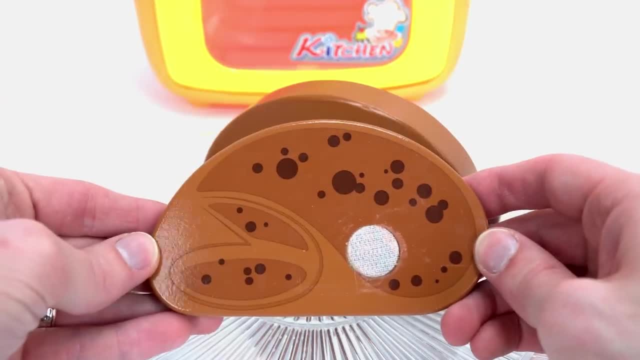 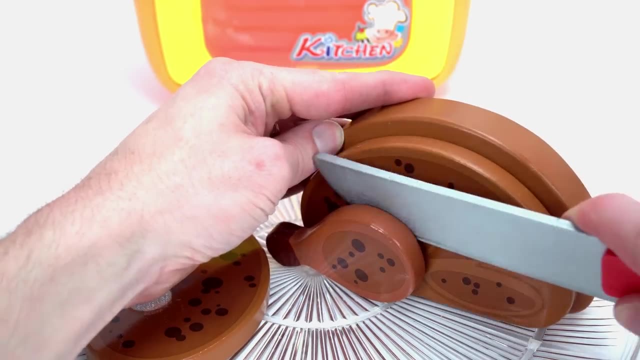 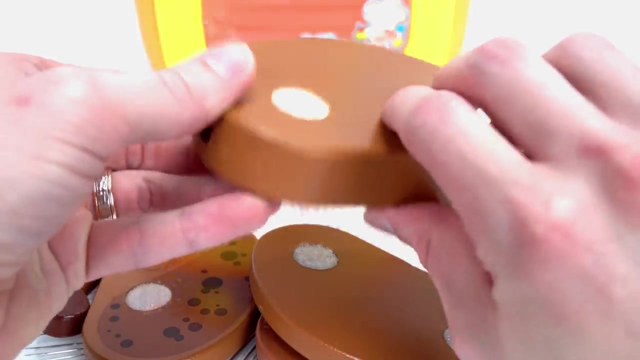 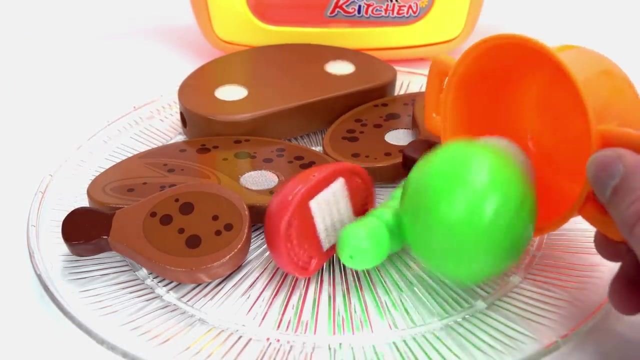 It довольно shielded it. This is a thigh. Everyone be careful, because this is you and me making stews. And here's the breast. Now our vegetables are done, Let's Strawberry. Add 나물, Add 나물. 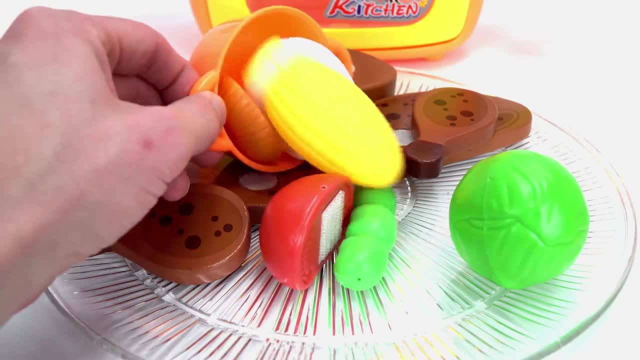 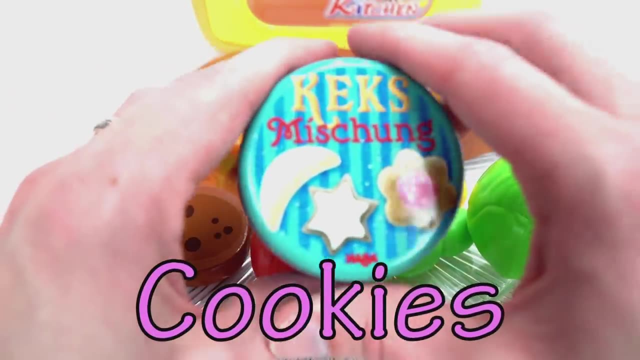 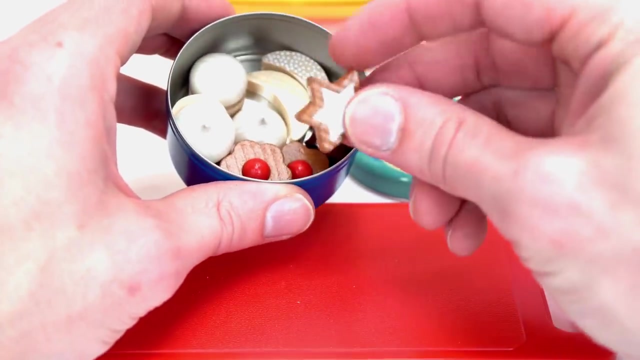 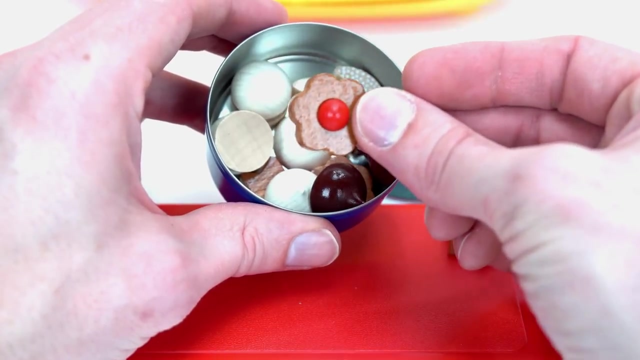 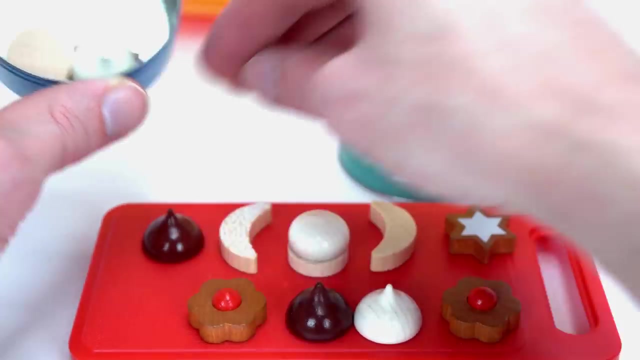 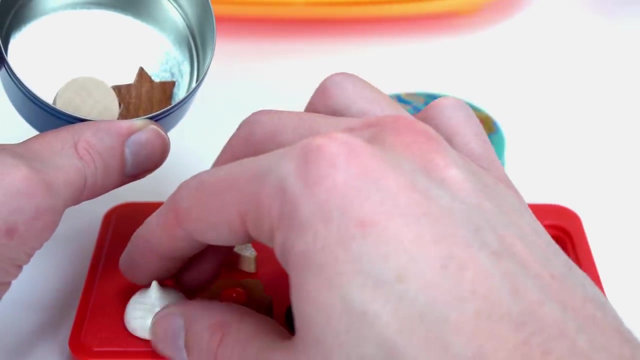 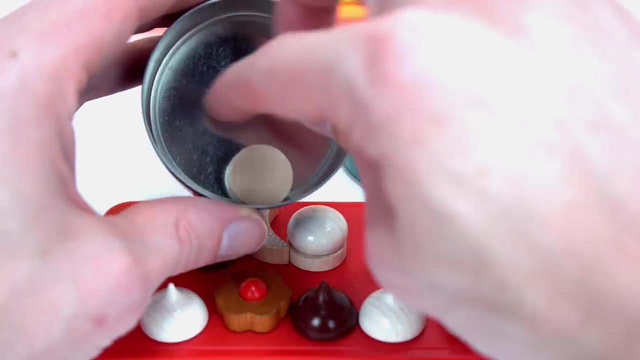 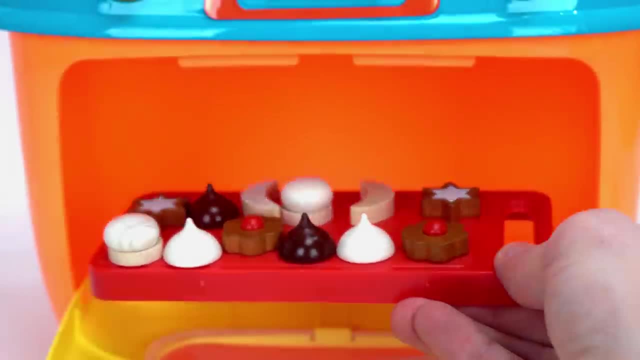 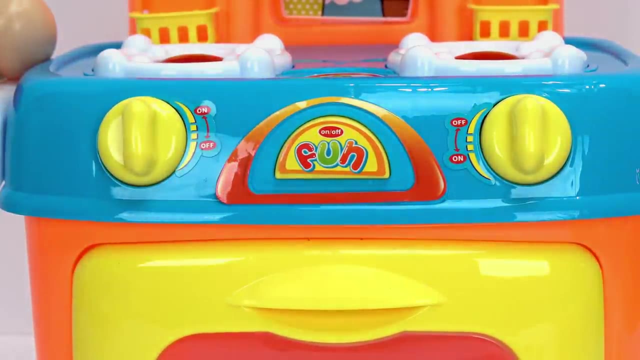 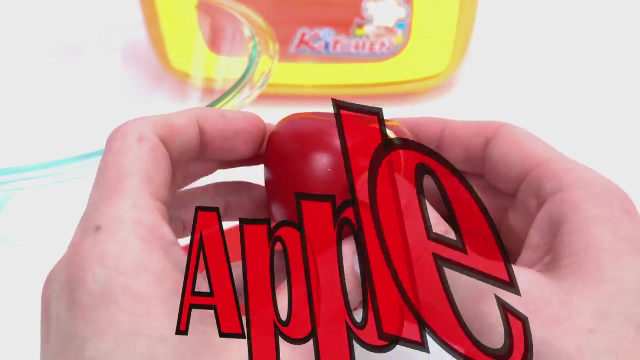 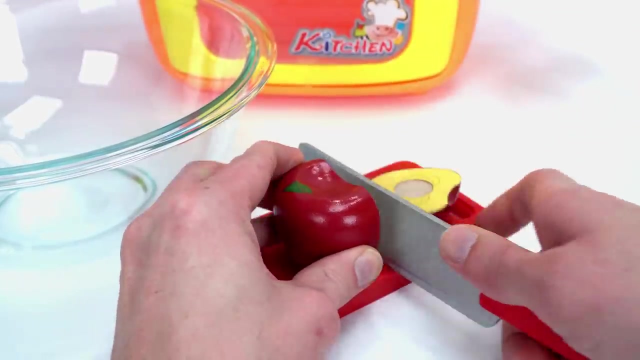 Let's pop these in the oven While they're baking. let's make a fruit salad. First, let's add an apple, Oh, Oh, Yummy. Here's a pear, It's nice, and green Watermelon, my favorite. 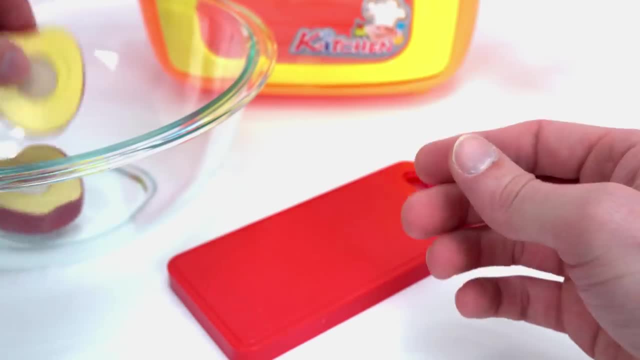 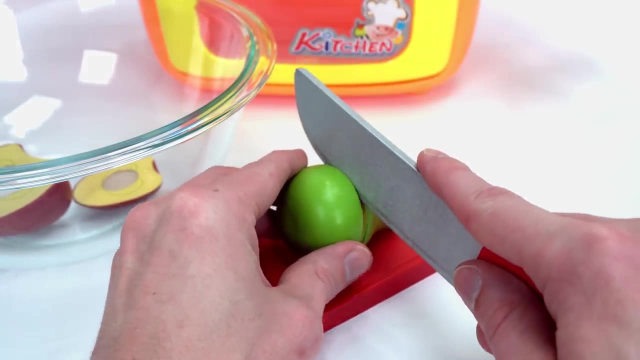 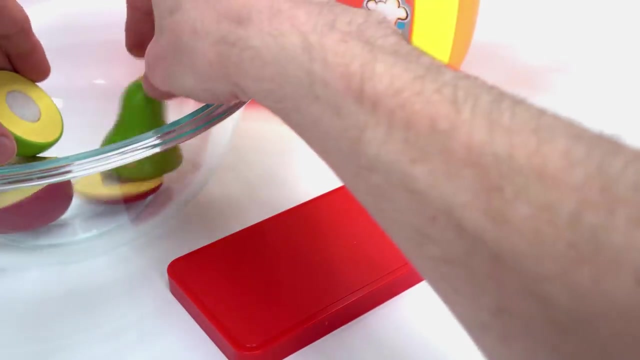 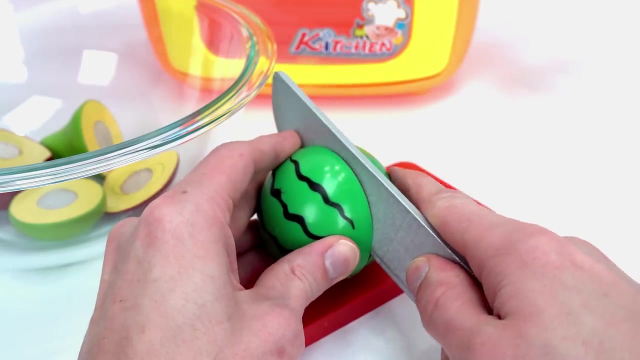 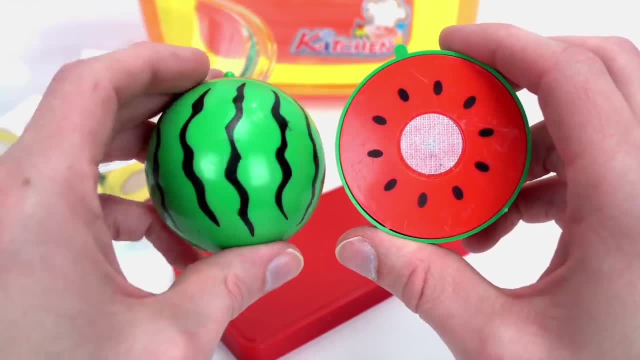 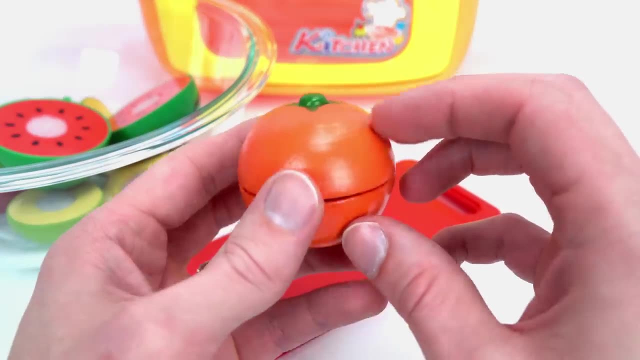 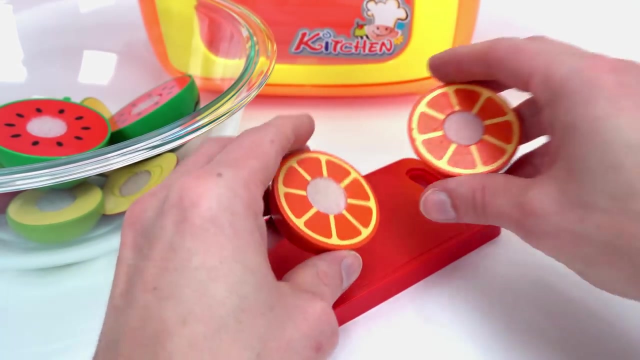 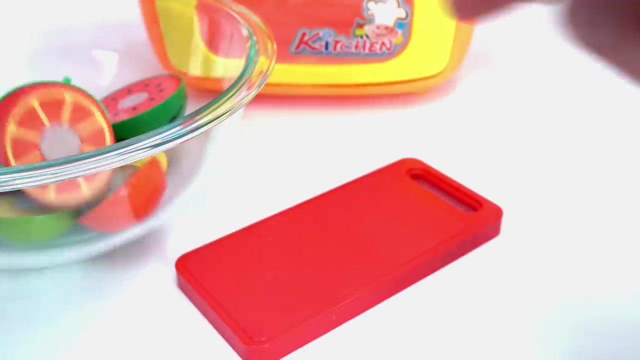 Oh, Oh, Oh, Oh Yeah, Oh, Oh, Oh Ooh. My eating skills are much better now. What is you'd like to share with me in the comments? Thank you, Awesome Nice yellow banana. These are so good for you. 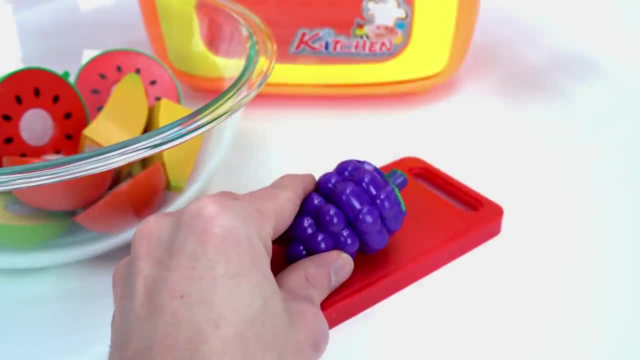 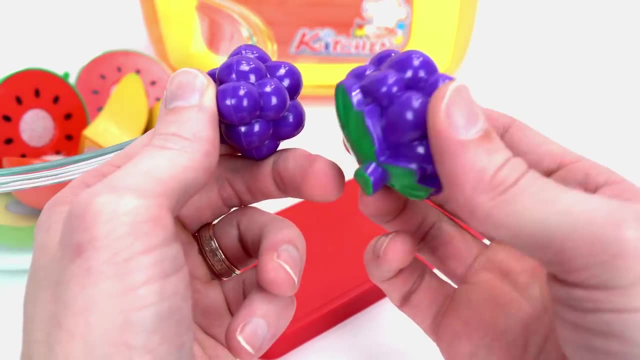 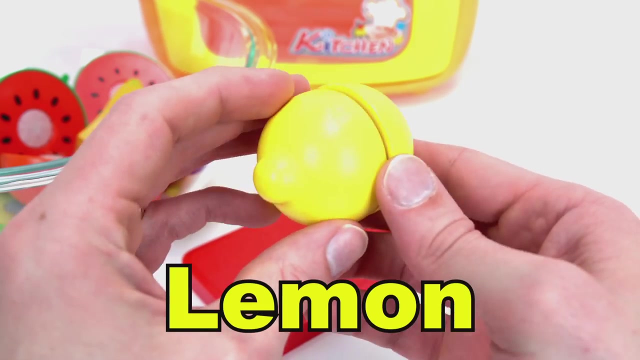 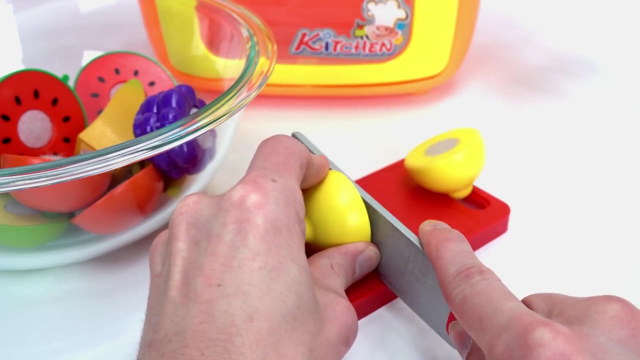 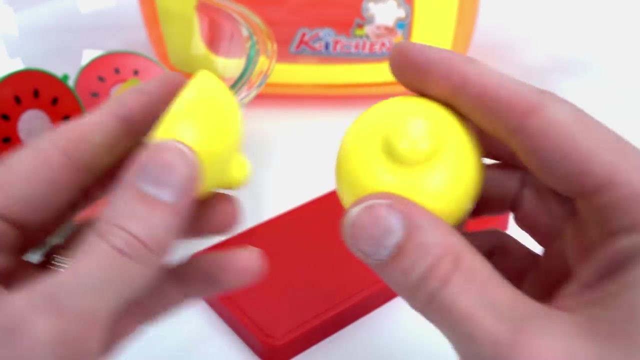 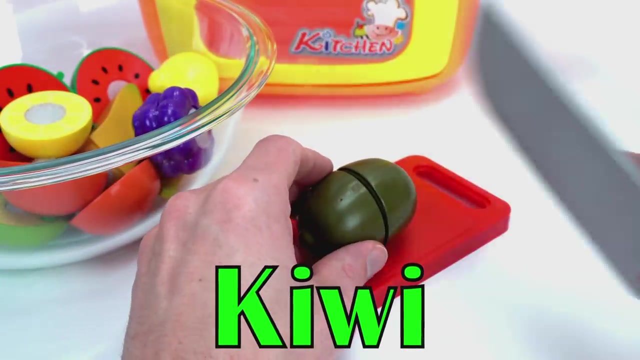 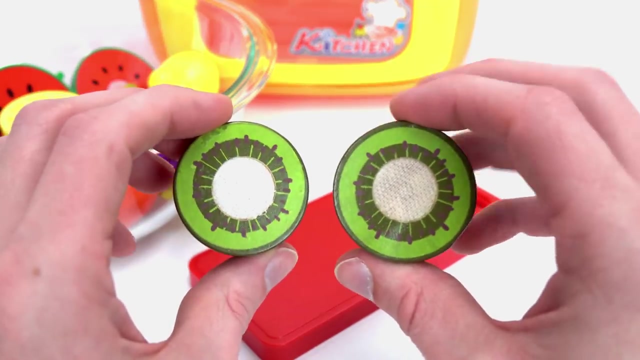 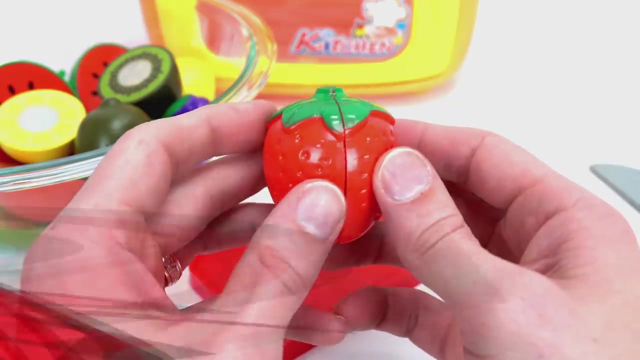 Here's some purple grapes. In you go. I like things a little sour, so here's a lemon. Do you know what this is? It's a kiwi. They're so yummy, You should try one. And finally, let's add a strawberry. 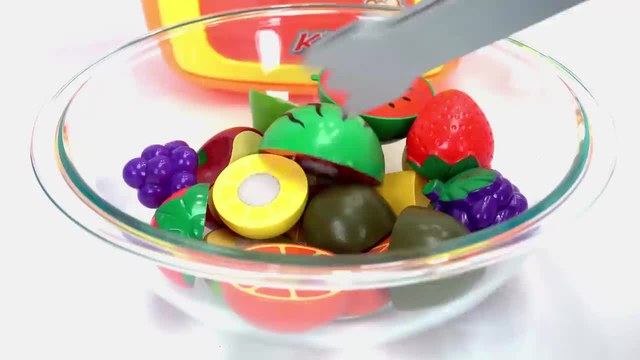 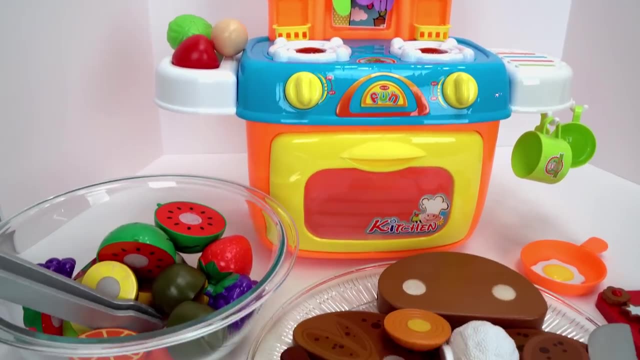 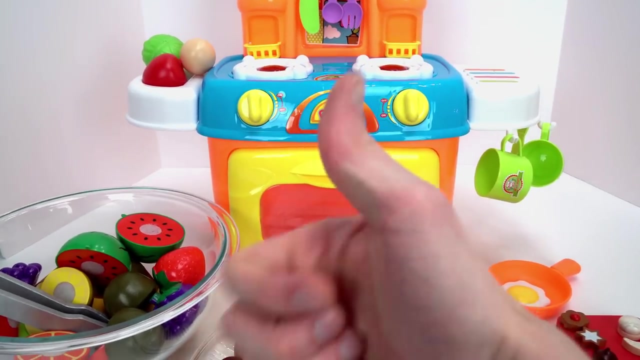 Now our fruit salad is perfect. Our cookies are done. Whoa awesome. Look at all this awesome food. Are you hungry now? Yeah, me too. Let's dive in. Give us a thumbs up if you like this video. Thanks for watching.